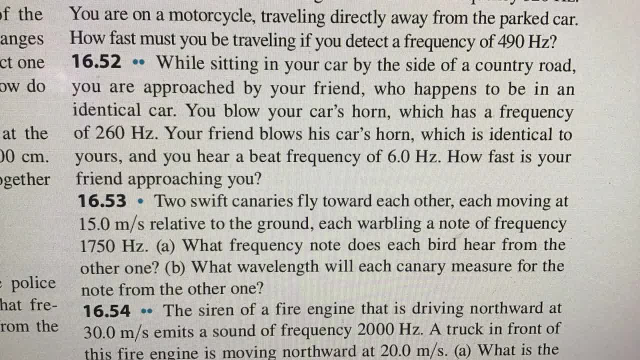 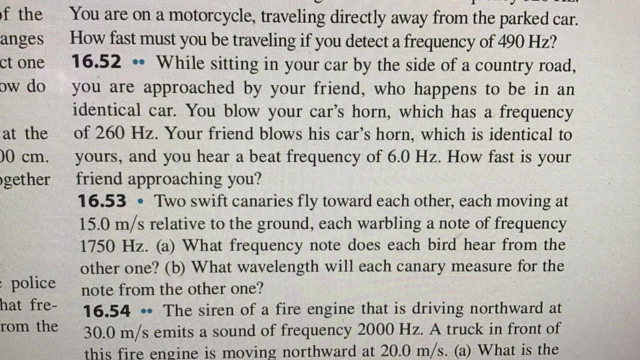 Okay, in this video we're talking sound, sound waves, sound effects, Doppler effect and something called beats. So we're taking in a good few of the topics that you learn about when you learn about mechanical waves, then learn about sound and so on. So we're looking at problem 1652. 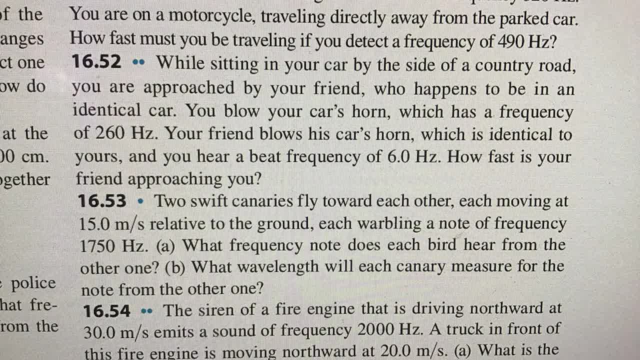 from Jung and Friedman. So, while sitting in your car by the side of the road, you're approached by your friend, who happens to be in an identical car. You blow the car's horn, which has a frequency of 260 hertz. Your friend blows his car's horn, which is identical to yours, and you hear what's. 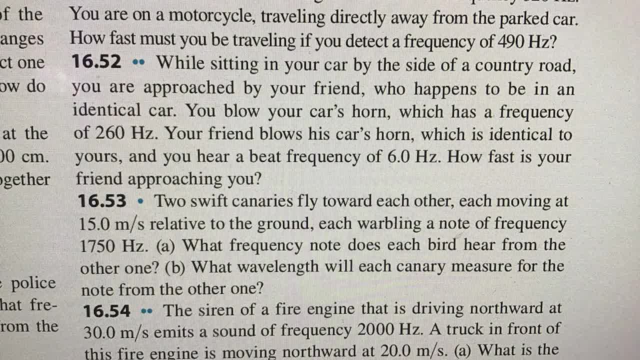 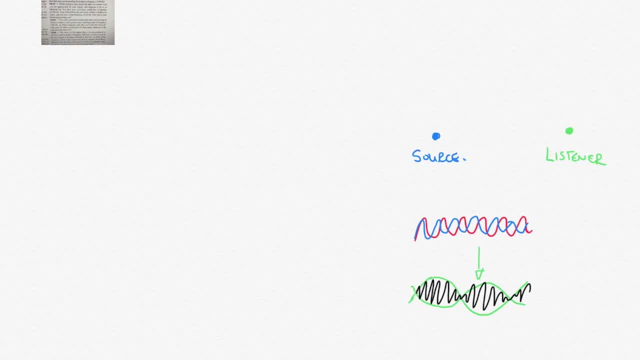 called a beat. frequency of six hertz- How fast is your friend approaching you? So first of all, we need to do a little bit of revision on what beats is. So beats is when you've got two waves that are quite close in frequency, overlapping with one another. they interfere with each other. 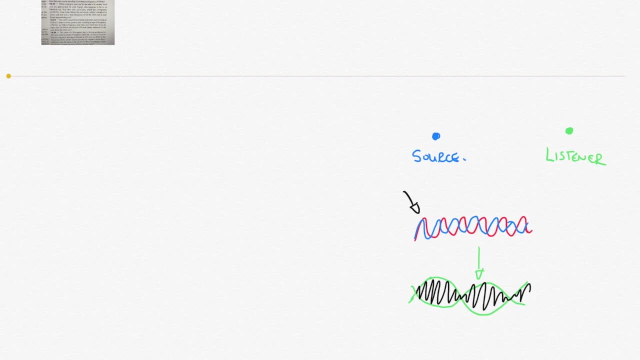 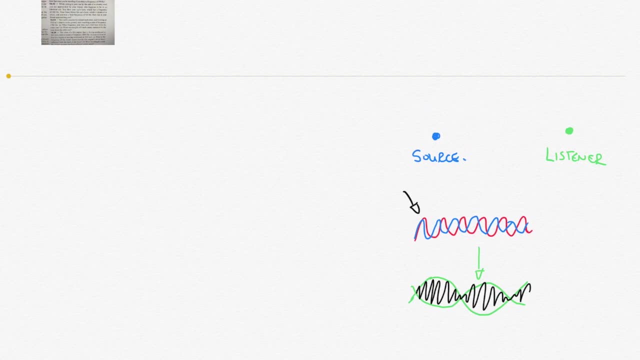 when we superimpose those waves on each other, we get something like what we have on the bottom, there, where we have this kind of pulsing wave here And the beat frequency is this frequency here. So it's the distance between these two nodes on this superposition of these two waves. 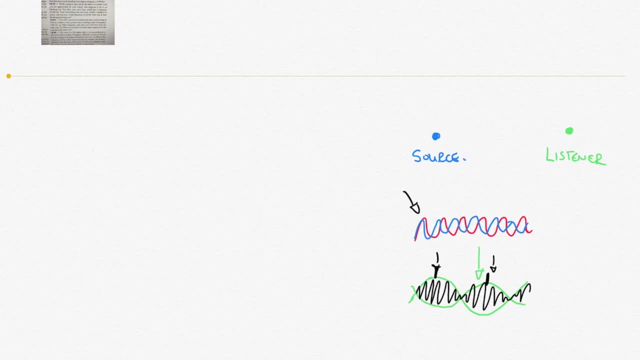 So if we've got two car horns operating at the same frequency, so the frequency here- F car we'll call it- is equal to 260 hertz. So the listener, he's emitting 260 hertz. The source is also emitting a frequency of 260 hertz, But the problem has told us that the source 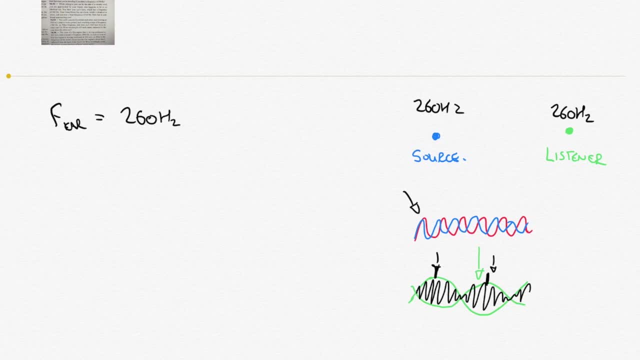 is moving towards the listener, So you're stationary in your car, emitting a sound or a frequency of 260 hertz. Your friend is moving towards you And, because of the Doppler effect, that is going to result in a frequency of 260 hertz, So you're emitting a frequency of 260 hertz. 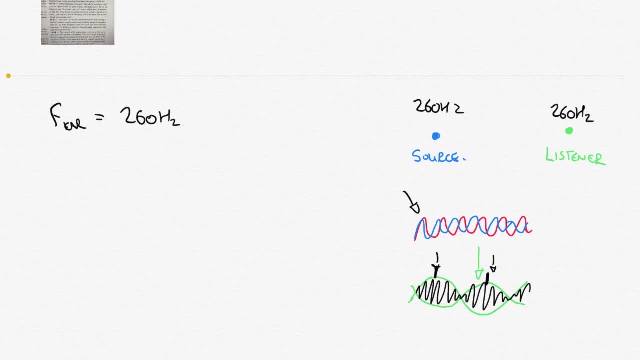 In an increased frequency, as observed at the point of the listener. So that you know, when you've studied the Doppler effect you see that the waves kind of bunch up and that results in an increased frequency. So that increased frequency is going to mix, if you like, or 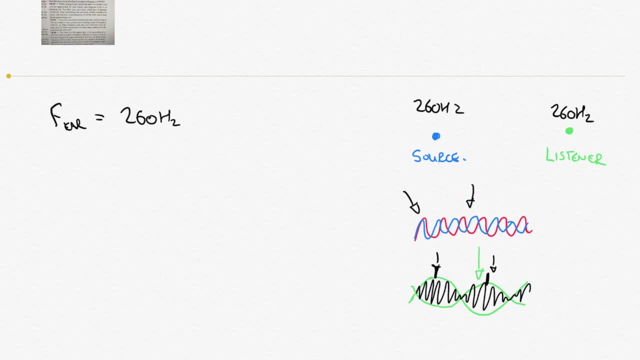 interfere with the regular 260 hertz frequency that the listener is emitting And they're going to cause a beat wave. And then what we've said is that the beat frequency, or the beat wave frequency is, is six hertz. So if we know a little bit about the Doppler effect and we know a little bit about 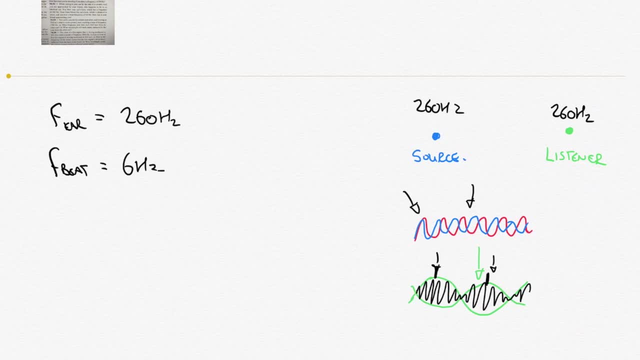 beats, we should from there be able to figure out how fast the car is moving towards you. So we know from studying the Doppler effect that the frequency heard or observed by the listener is equal to the velocity of the sound wave plus the velocity of the listener divided by the 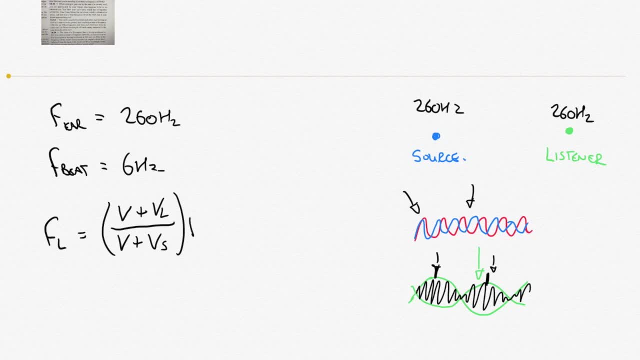 velocity of the sound wave plus the velocity of the listener, And that's going to result in a velocity of the sound wave plus the velocity of the source multiplied by the frequency of the source. So the apparent frequency recorded by the listener is equal to the velocity of the wave plus. 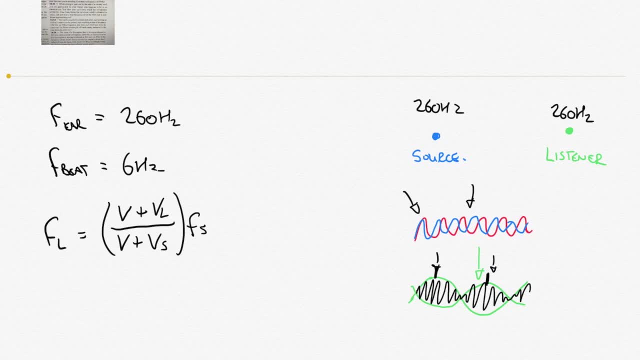 the velocity of the listener divided by the velocity of the wave plus the velocity of the source, all multiplied by the frequency of the source. Okay, So in this case we can get rid of one term, because we know that the listener is not moving. So this velocity here is zero And our 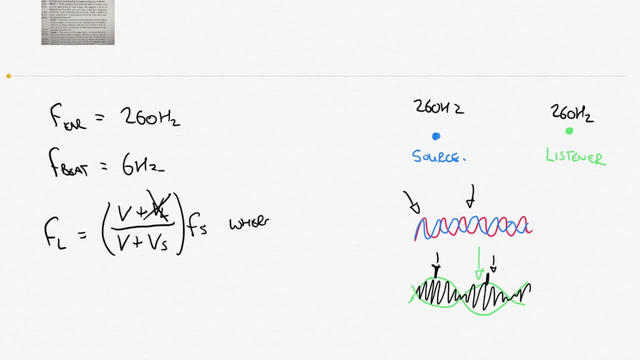 equation is slightly simplified And we also know that, and we'll just change the notation here- the frequency of the source is 260 hertz. So there we go Now. the beat frequency is going to be the difference. So when we study beats, we find out that the beat frequency is going to be the difference. 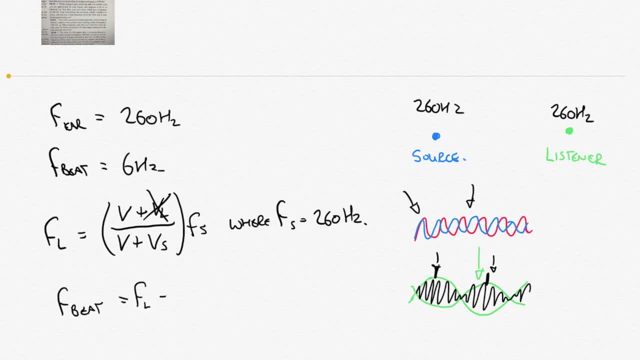 in frequency between the two waves. So it's going to be the frequency that the listener sees, minus the frequency of the source. So we have a beat frequency of 6.0 hertz, 6.0 hertz. So what that tells us then is that the beat. 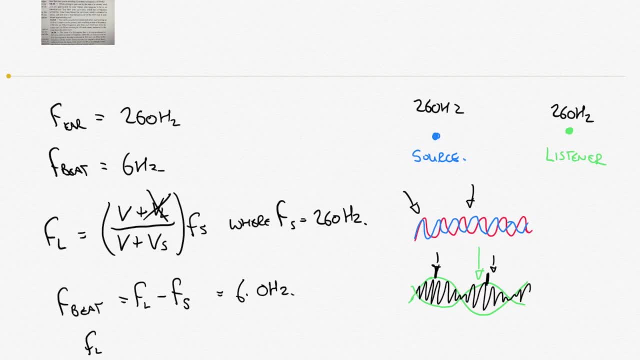 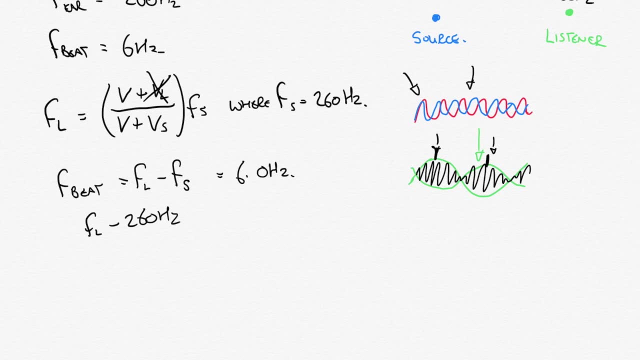 frequency is going to be equal to the frequency of the listener minus 260 hertz. So the frequency, remember, of the source is 260 hertz, which is what we've put in here. So just make this link between these two here And that's going to be equal to oops, back to black, That's going to. 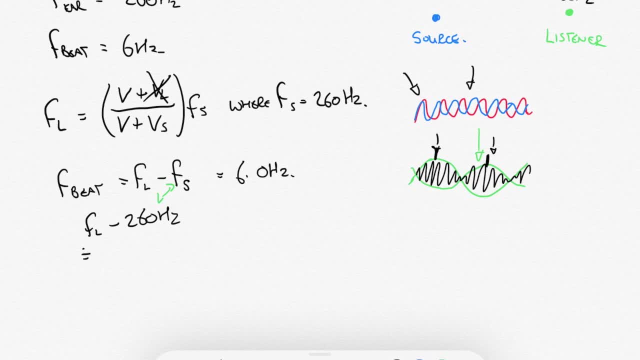 be equal to the frequency of the listener minus 260 hertz. So that's going to be equal to the 6.0 hertz. Okay, So what that tells us, then, is that the frequency heard by the listener is 266 hertz, So the beat frequency is 6.0.. The source frequency is 260.. So the frequency that the 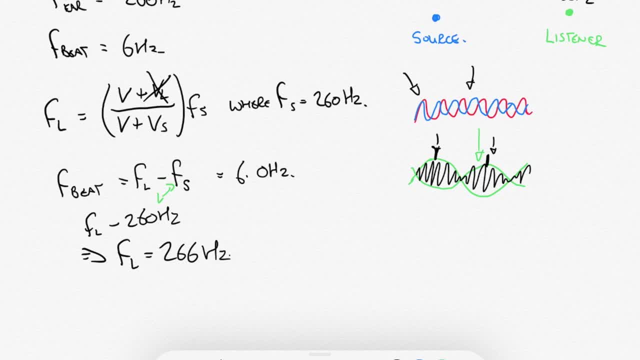 listener observes now is 266 hertz. So now we can plug this into the equation, the Doppler effect equation. So we have- let's go to red here. We have the frequency that the listener hears. now We can know the velocity of the wave, because it's a sound wave in air. So it's going to be. 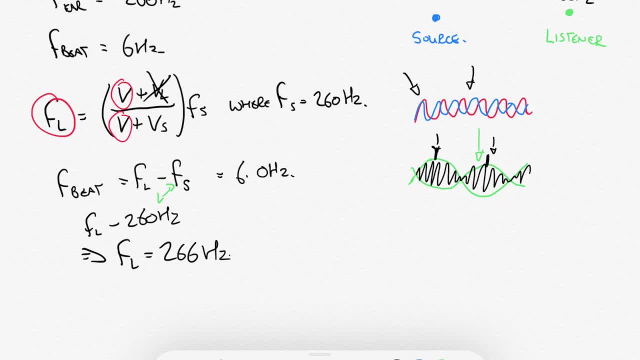 344 meters per second, which is what we take for the velocity of a sound wave in air, And we know the frequency of the source is 260 hertz, which is given to us in the question And the only unknown. then, in our Doppler effect equation is for the velocity of the source And 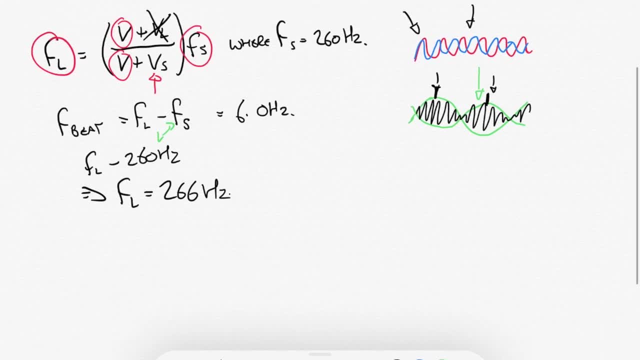 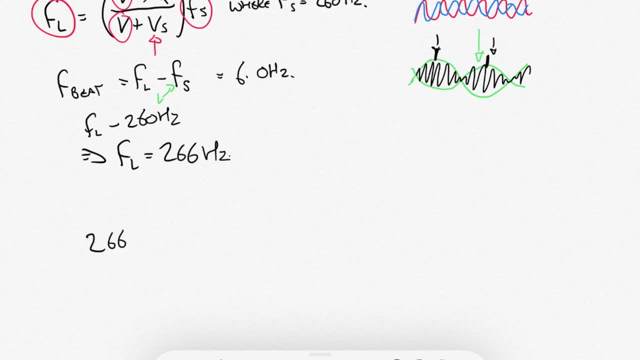 the velocity of the source is exactly what we're um setting out to measure. Okay, So let's plug in what we have for the equation. So velocity- sorry, a frequency for the listener. 266 hertz equals velocity of sound. 344 over the. 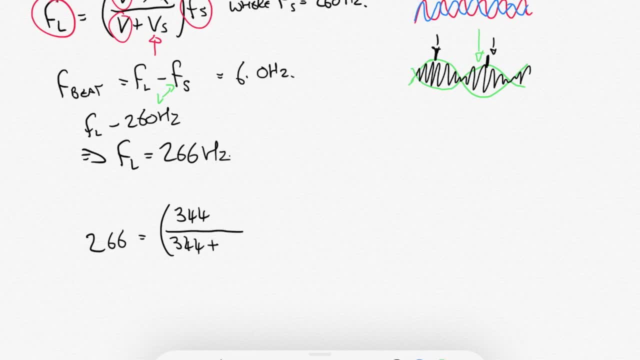 velocity of the sound plus the velocity, or sorry, the- yeah- the velocity of the source, which is what we're trying to solve for, isn't it? Yeah, So the velocity of the source all multiplied by the frequency of the source, which is 260 hertz. 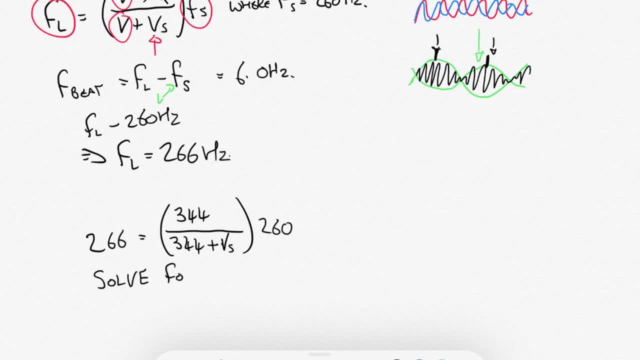 So solved That then? so let's say, solve for Vs velocity of the source, And that gives us- let me just check this one out- That gives us minus 7.8 meters per second. So what that tells us is that the 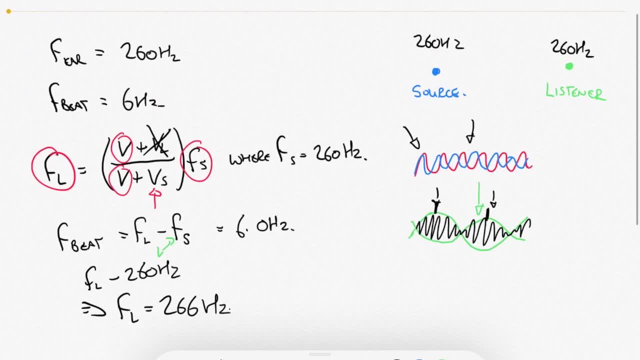 source is moving towards us at 7.8 meters per second. So then, if we look at that in the context of the source, we can see that the source is moving towards us at 7.8 meters per second. So that's the velocity of the listener. So we have the velocity of the listener, So we have the. 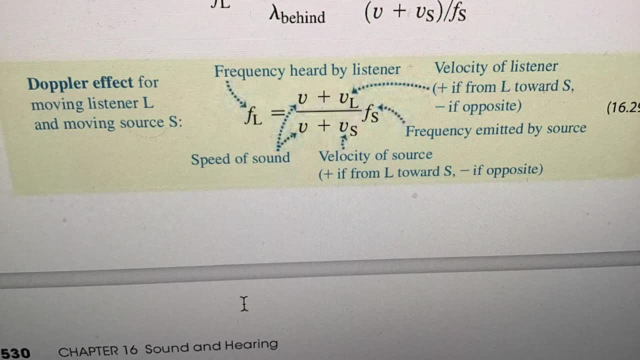 equation for the Doppler effect that we see in the textbooks. So we have um V plus VL. So VL is the velocity of the listener and the sign conventions in the way this equation is derived is that the velocity of the listener is going to be positive if the motion is from the listener towards the.